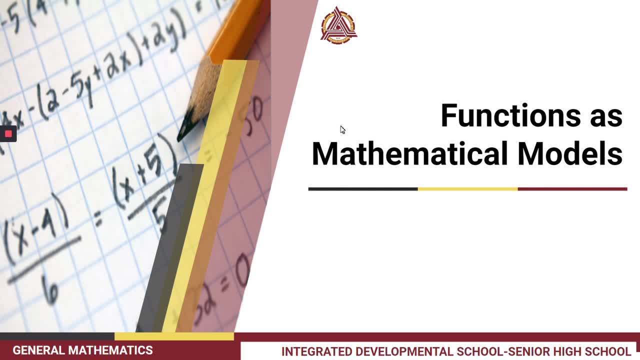 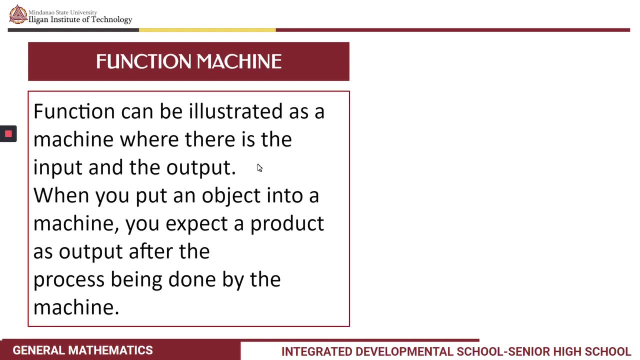 the. So before we proceed with examples, real-life examples in which we can associate functions, let us define function-machine first. Function can be illustrated as a machine where there is the input and the output. When you put an object into a machine, you expect the product. 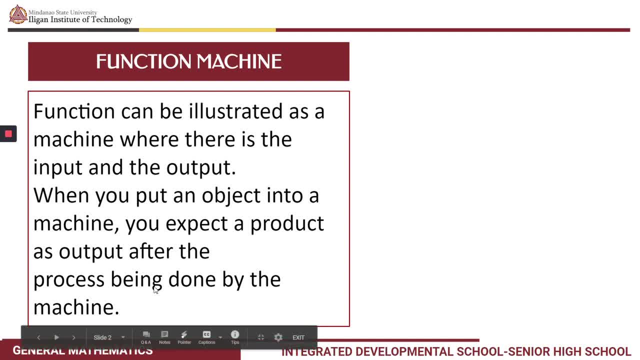 as output after the process being done by the machine. So in this figure, basically this definition of function-machine is just the definition also of our function as itself. I have discussed that in function we can call a relation a function if and only if, one input can only generate one output, not two or more. 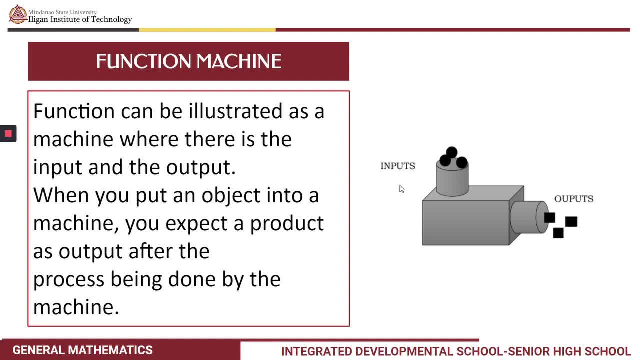 so in here, in our machine, function machine, it says that let's say we have input if we put something on the machine, in the machine and then with that, with whatever rule that that the machine it has is, will have an output, only one output. we can't have two or more output. say, for example, we put orange in the 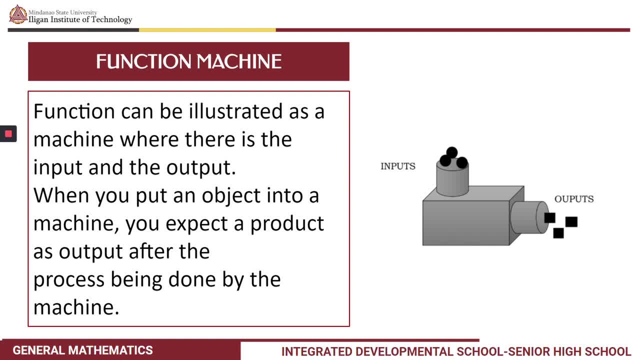 juicer. no orange fruit in a juice juicer, so we would expect that the outcome is an orange juice. no, we can't have an outcome which is a grapes or orange and grapes juice, because you only put orange in that machine, which is what the machine I'm talking about is: the juicer. okay, 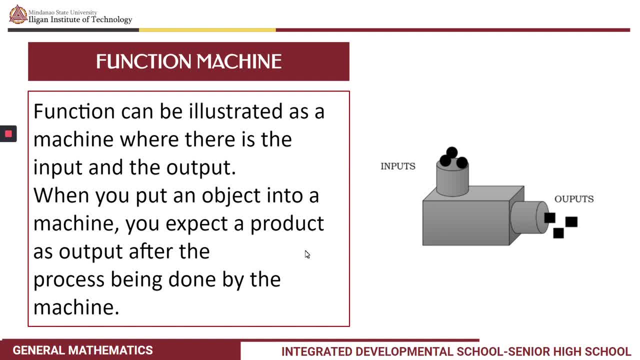 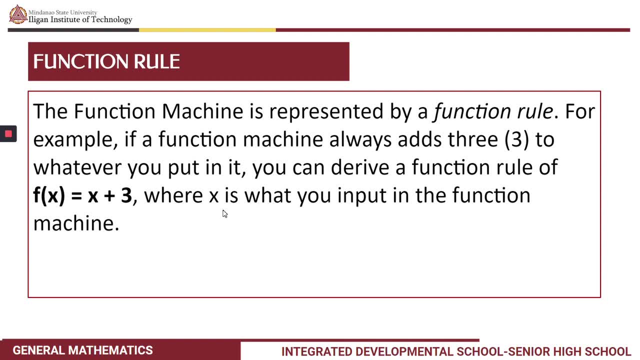 so how do we make a function model so the function machine is represented by a function rule? for example, if a function machine always adds 3 to whatever you put in it, you can derive a function rule of f of X equal to X plus 3 where X is. 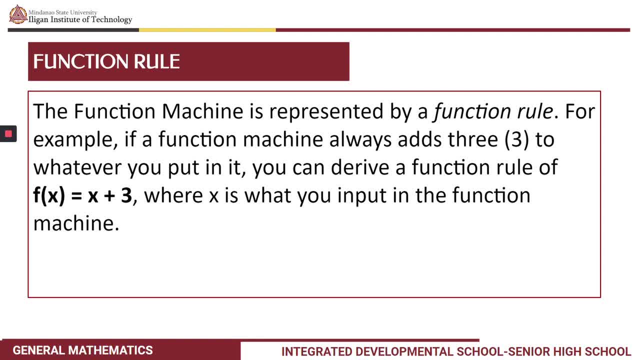 what you input in the function machine. so for example, now this one, so the in here- has a function rule which is: it always adds 3 to whatever you put in it. so that is why we'll have a function rule which is f of X equal to X plus 3. 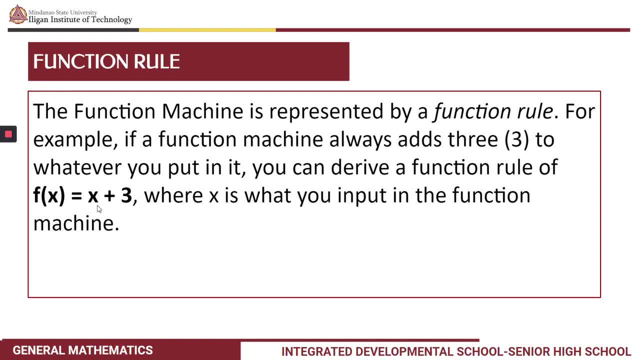 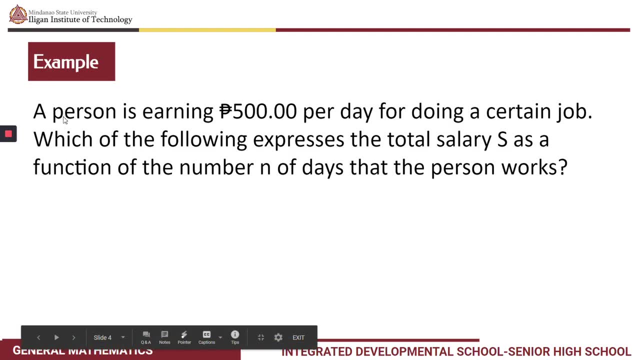 in which X is the input and f of X is the output. okay, so that is how we we make our representations. no for the function machine. okay, so say. say, for example: now we have a person which is earning 500 passes per day for doing a certain job, which of the following expresses the total salary as: 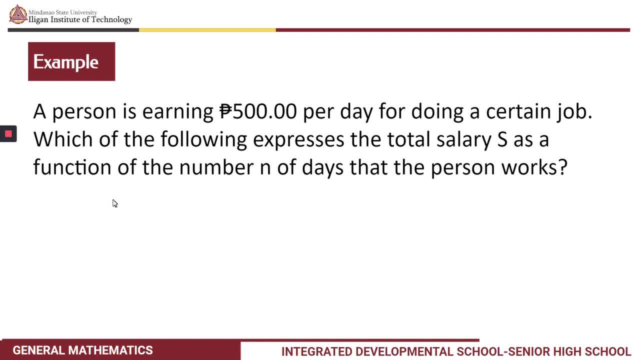 a function of the number of n of days that the person works. so in generating a function rule or in trying, when you try, to model a particular situation, you need to identify what is the input or the independent variable first, and also the dependent variable or the output. so in this case, what do you think is the input? yes, it is. 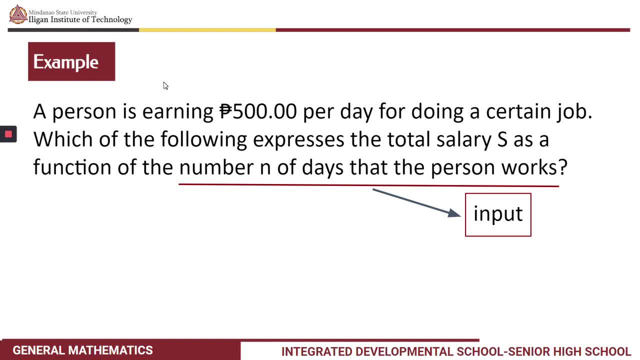 the number of days that the person works, all right, and the output, of course, is the total salary that the person will be getting. so you already have your input. the next thing that you need to do is to observe the situation. what is the rule here? the rule here is that a person is earning 500 pesos per day, so it's 500. 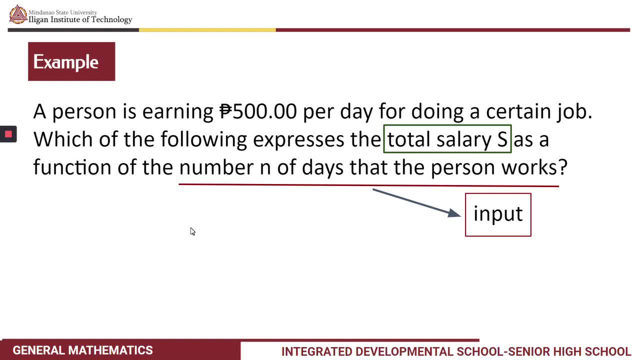 pesos per day. so that is why your representation now it will be s of n equal to 500, n, or 500 times n, in which n is your number of days that the person work and s of n is your number of days that the person works and s of n is your. 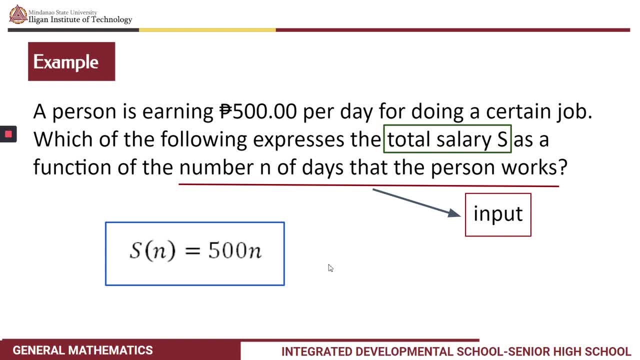 number of days that the person works, and s of n is your number of days that the person will be getting. so it's that simple. so what do you think is the domain? okay, we have here. domain is from 0 to positive infinity. why? because we cannot have 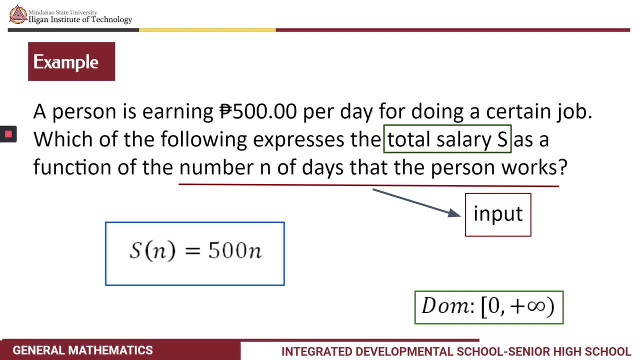 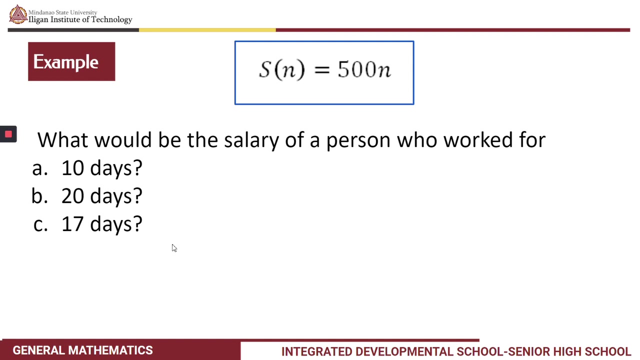 negative n or negative number of days. right, we count from 0 to 3, so our domain is from 0 to positive infinity. Okay, so this is just an easy example. so let's try to solve how much the person will be earning if he or she will work for 10 days or for 20 days and for 17 days. 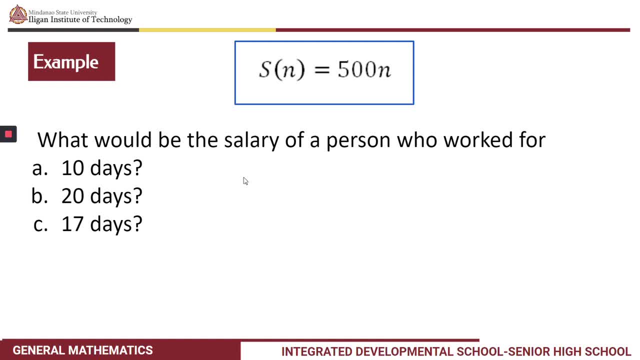 So to solve that it's actually very easy. You just have to evaluate the function using these values. So first let's try to solve for 10 days. You just have to substitute n with 10.. So we have S of 10, equal to 500 times 10.. 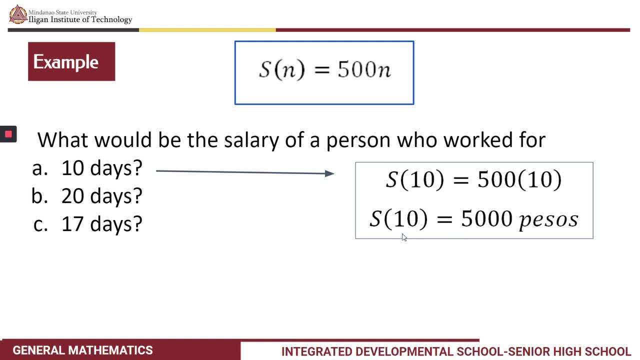 So that is why the person will be getting 500 pesos. if the person will work for 10 days, How about 20 days? You just have to substitute 20 to n and then you'll find 10,000 pesos. You'll be able to solve for 10,000 pesos. 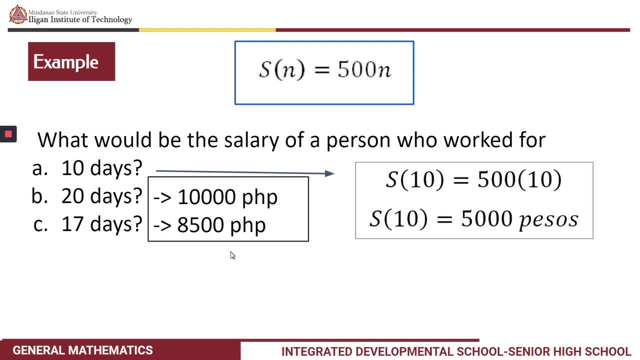 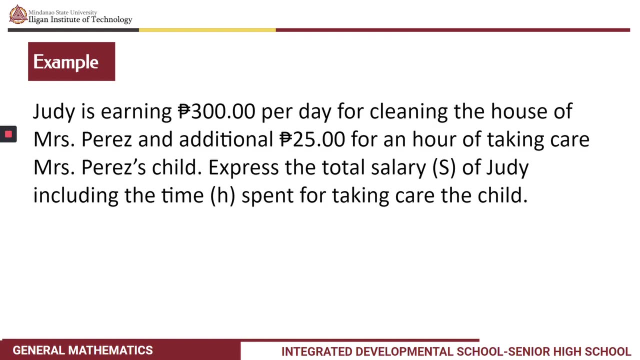 And then for 17 days. Okay, You have 8,500.. So that's how we model real life situations using function. So let's have another example: Judy is earning 300 pesos per day for cleaning the house of Mrs Perez, and additional 25. 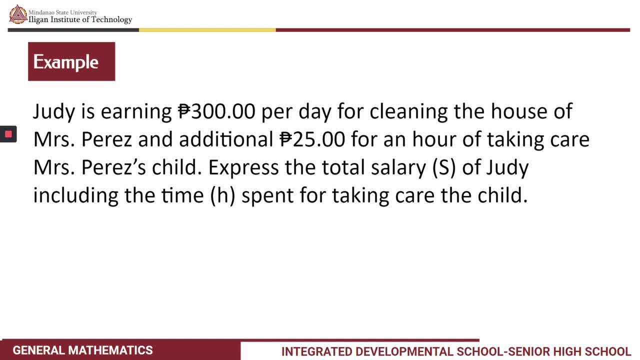 pesos for an hour of taking care of Mrs Perez's child. Express the total salary. What is the total salary of Judy, including the time age spent for taking care of the child? Okay, So what do you think is the domain, or the input, or the independent variable here? 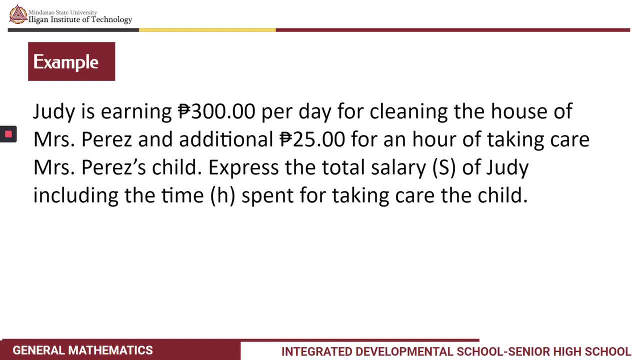 It is the time Judy spent taking care of the child, And the output here is the total salary S. Okay, So that's the output. Next thing to do is to observe the situation and generate a function rule. What do you think is the? what do you think will be the function rule? 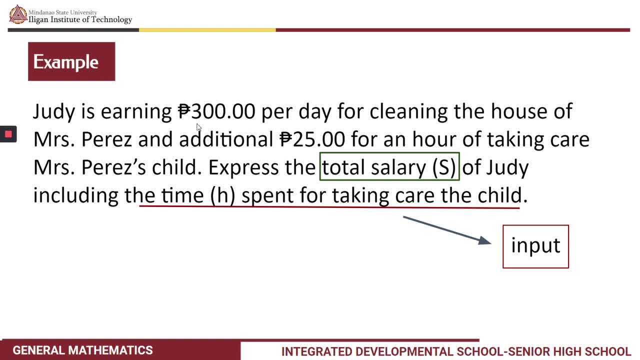 See, you have 300 pesos per day. So here we have 300. Plus, if Judy will take care of Mrs Perez's child, Okay, She'll get 25 pesos per hour. So that's why we have S of H equal to 300 plus 25 H. 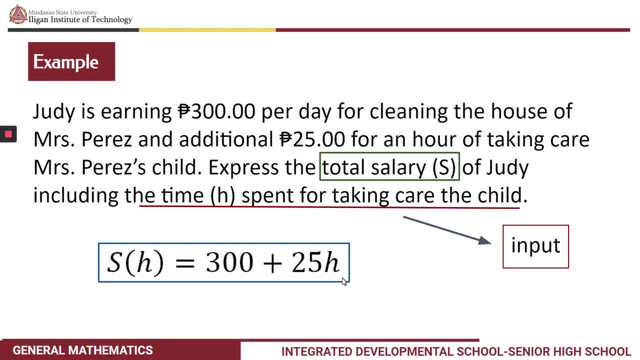 Where H is the number of hours Judy spent taking care of the child, And 300 here is her pay for cleaning the house. So that, so this is the model of this situation. Okay, So what do you think is the domain of this function? 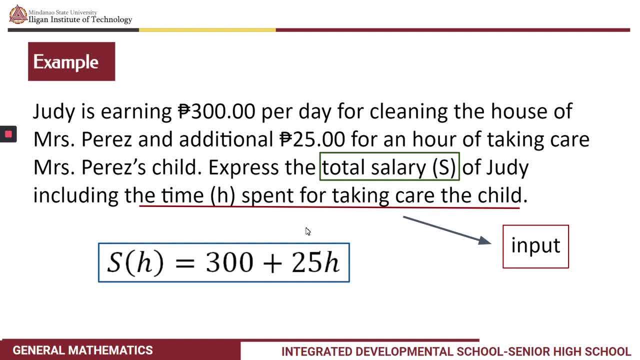 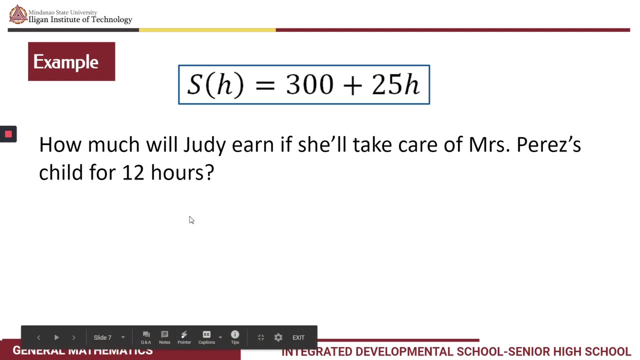 So H can only take zero non-negative right, zero to the positive infinity, same. no, because we have- we don't have- negative number of hours, So let's try to solve Okay. So how much will Judy earn if she'll take care of Mrs Perez's child for 12 hours? 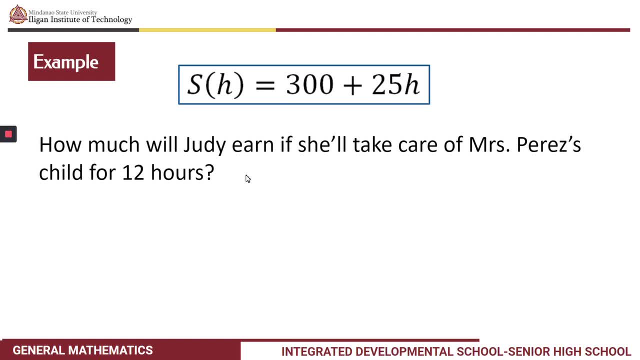 Simple. You just have to substitute 12 for H. no, So we have S of 12 is equal to 300 plus 25 times 12. And if you solve that accordingly using Jamdas, you'll get 600 pesos. So Judy will be getting 600 pesos. 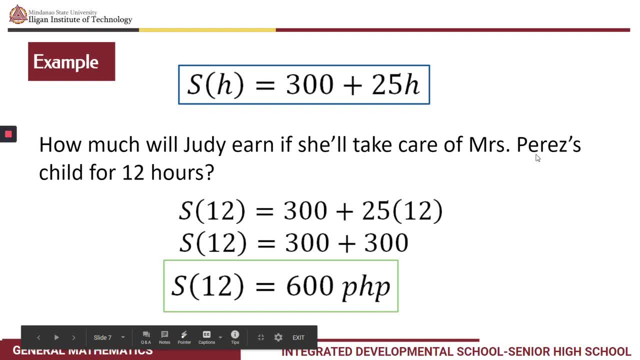 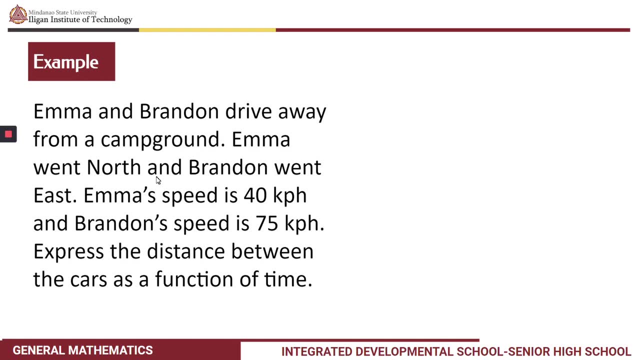 Okay, Okay, She's taking care of Mrs Perez's child for 12 hours. So easy, lalang, no. So it's simple. Let's try another example. This one: Emma and Brandon drive away from a campground. Emma went north and Brandon went east. 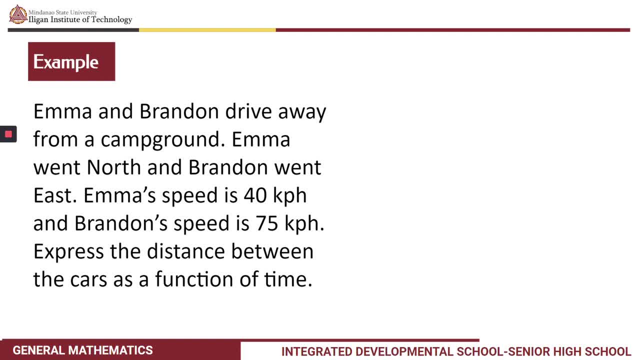 Emma's speed is 40 kilometers per hour And Brandon speed is 75 kilometers per hour. Okay, Express the distance between the cars as a function of time. Ayan, So the situation is like this. So they came from the same campsite or campground. 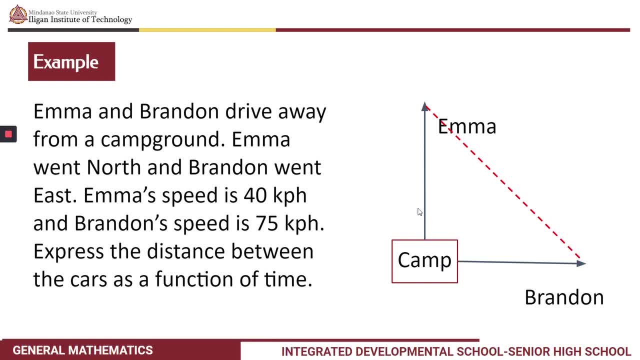 And then mag-separate na sila. no, Si Emma papuntang north, si Brandon papuntang east naman. So we are looking actually for the distance between the two cars. no, Emma's car and Brandon's car. 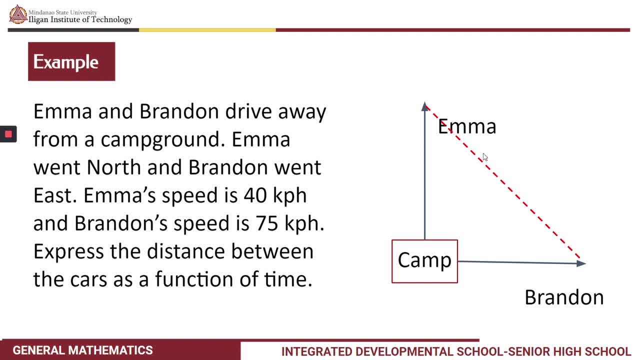 So this red line here represents the distance between Emma and Brandon. Familiar ba yung figure? Yes, no, You were able to make a right angle triangle, no Right triangle. So when we say right triangle, anong nasa isip natin? 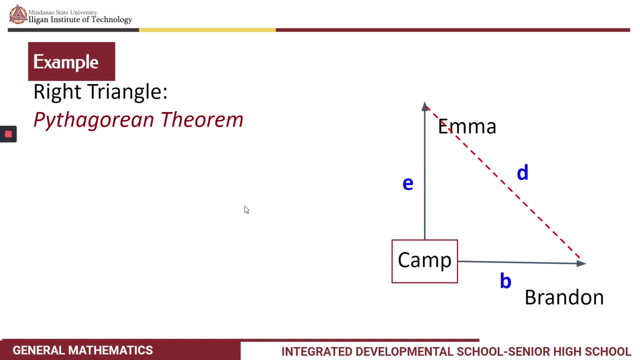 Right triangle Pythagorean theorem. So I believe, I hope, that everyone is familiar with Pythagorean theorem. So let's say E is the distance covered by Emma and B is the distance covered by Brandon from the camp. D will be the distance between Emma and Brandon. 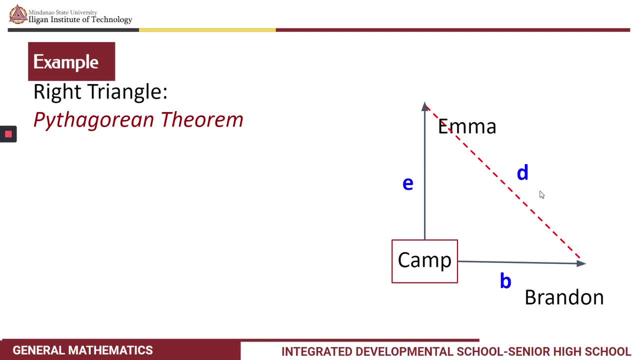 So how do we solve for D? Okay, Because we are looking for D here. With this, we'll have D squared equal to E squared plus B squared, using the Pythagorean theorem. Okay, So how can we relate it with our situation? 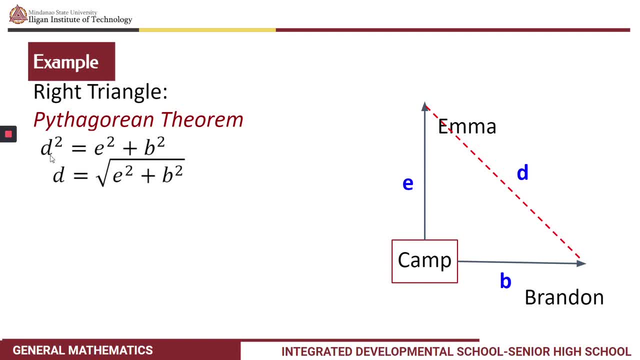 Okay, So we are looking for D, so we need to square root both sides, So we'll have square root of the sum of the squares of E and B is equal to D, which is the distance of Emma and Brandon. So how can we relate it with the situation? 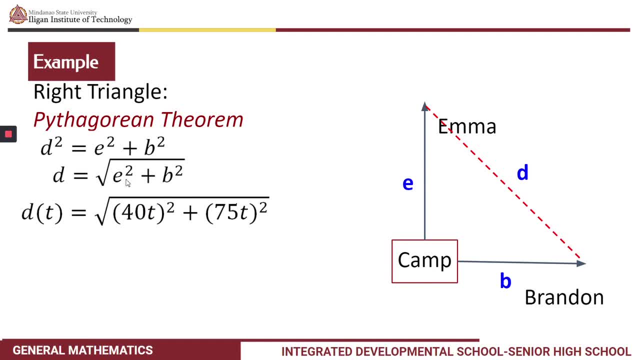 We know that Emma's speed is 40 kph. We also know that Brandon's speed is 75 kph, So that's why we need to substitute only no 40 T. What is T? T is the time, no. 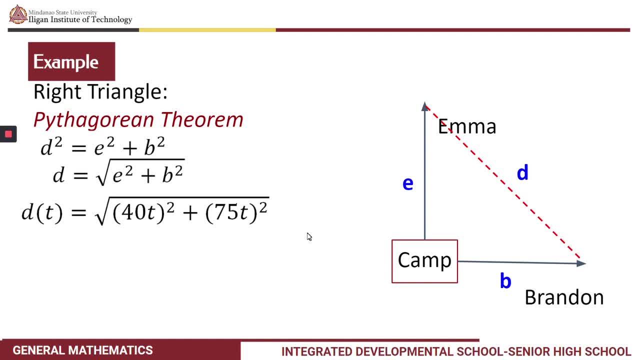 That Emma and Brandon drove no So. So in here, T is our input or our independent variable- the number of hours they're driving, And D of T will be the distance between Emma's car and Brandon's car. So if you are to simplify this one, 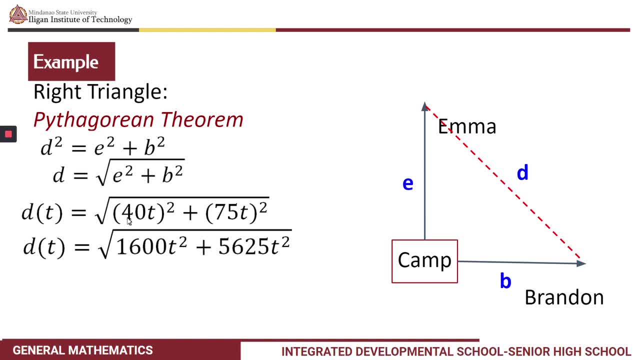 So the square of 40 T is 1600 T squared And the square of 75 T is 5625 T squared. So combined like terms you will get square root of 7,225 T squared, So is 7225, a perfect square. 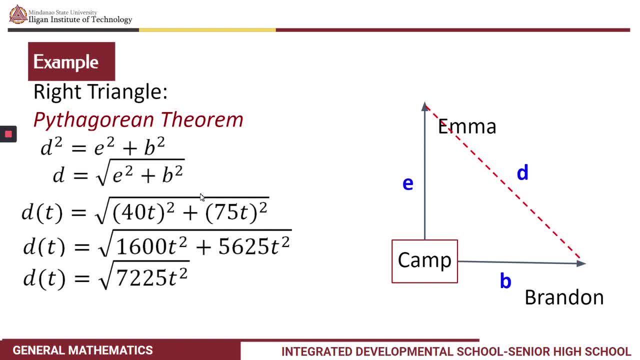 Yes, it is a perfect square And its square root is 85. So you'll have D of T equal to 85 T, Where T is the number of hours Emma and Brandon's driving And the D of T is the distance between Emma's car and Brandon's car. 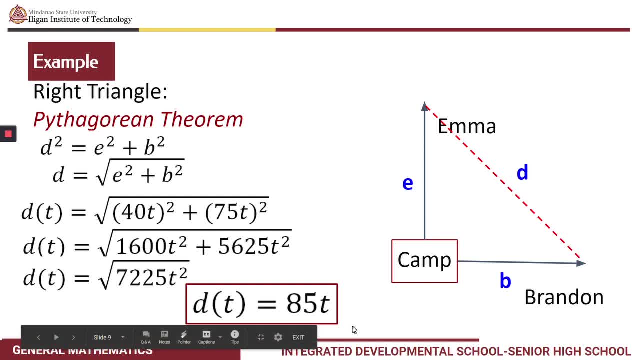 So you will use this representation or function. So if you're asked, let's say what's the distance between Emma's car and Brandon's car after 5 hours? you'll just have to replace T with 5.. So easy, right. 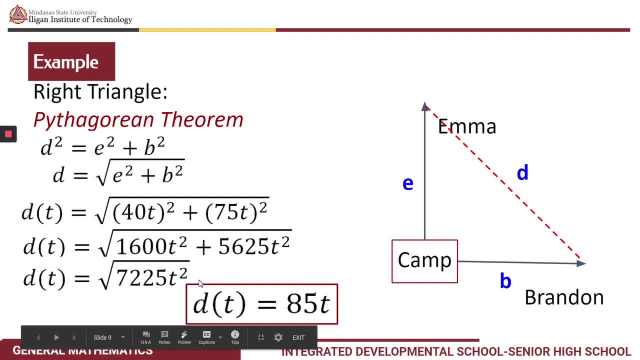 Yes, If you have this, you can solve. you can solve it directly. So that's the essence of functions as mathematical models. Okay, let's try. The domain also here is from 0 to positive infinity. Why? Because we don't have negative distance. 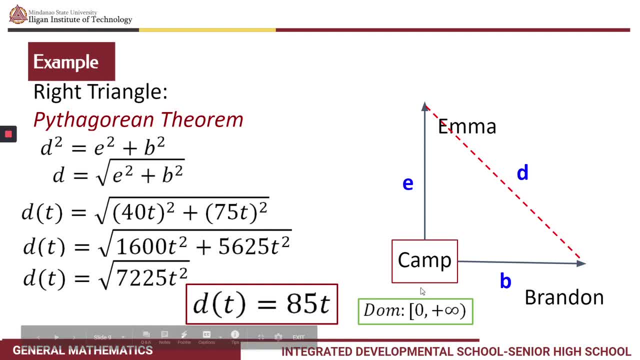 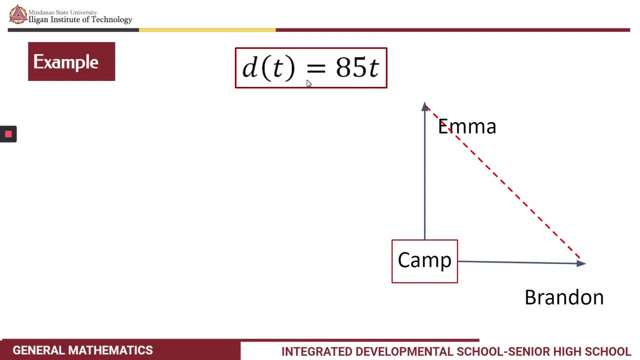 Everyone knows that right. Okay, So we already have the function rule or representation of the situation. So let's try to solve the distance between Emma's car and Brandon's car after 3 hours of driving. Okay, In solving we just have to substitute T with 3.. 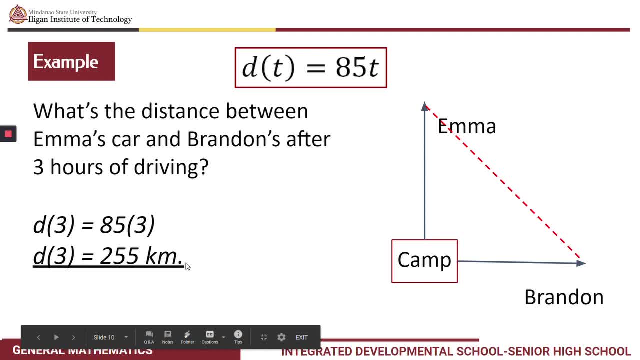 So you have D of 3, equal to 255 kilometers. So this will be the distance between Emma's and Brandon's car after 3 hours. So that's how easy it is. The challenging part is generating the function rule or the model. 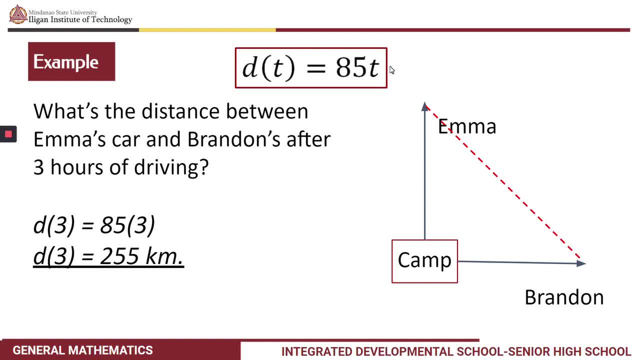 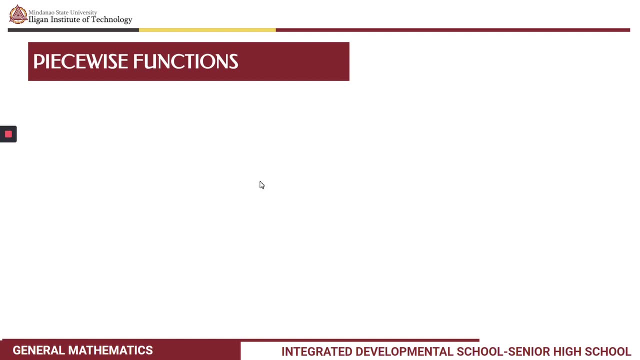 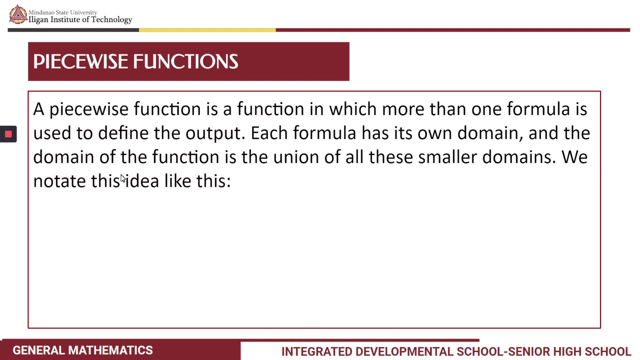 So when we solve, we just have to substitute. Okay So, yes, Okay. So we have another type of function, which is the piecewise functions. Okay, What are these piecewise functions? A piecewise function is a function in which more than one formula is used to define the 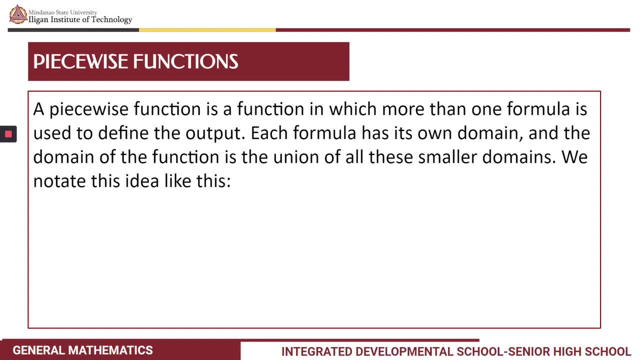 output More than one formula. Each formula has its own domain and the domain of the function is the union of all these domains. We we notate this idea like this: Okay, Let's say we have F of X, F of X equal to, let's say, formula 1, if X is in the domain 1.. 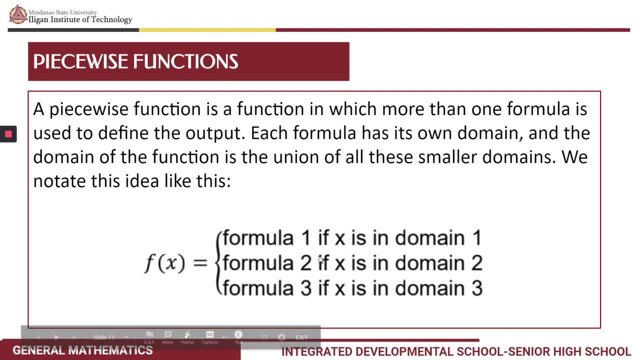 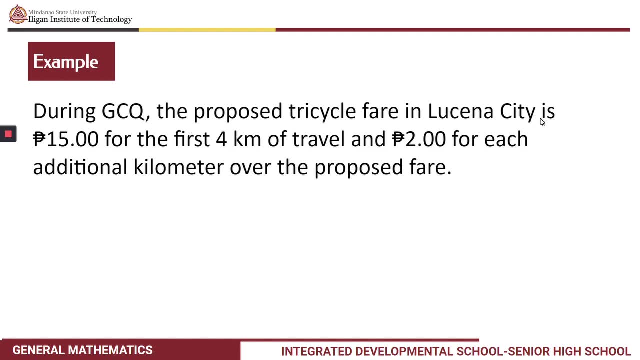 Formula 2 if X is in domain 2. Formula 3 if X is in domain 3.. Okay, For you to understand this better, let's have an example. During GCQ, the proposed tricycle fare in Louisiana City is 15 pesos for the first 4. 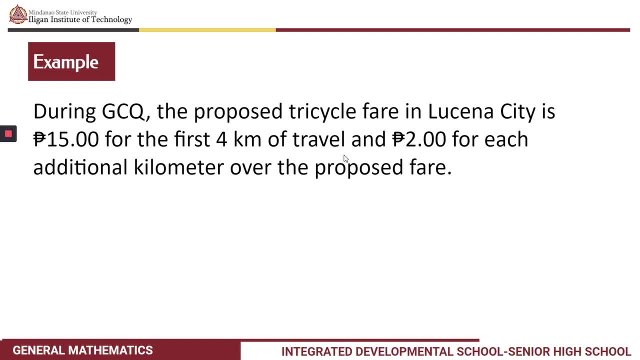 kilometers of travel And 2 pesos for each additional kilometer over the proposed fare. So ayan, So again, para makapagrepresent tayo ng function, para makagenuate tayo ng function rule or model for this situation, we need to identify the domain and the range first, 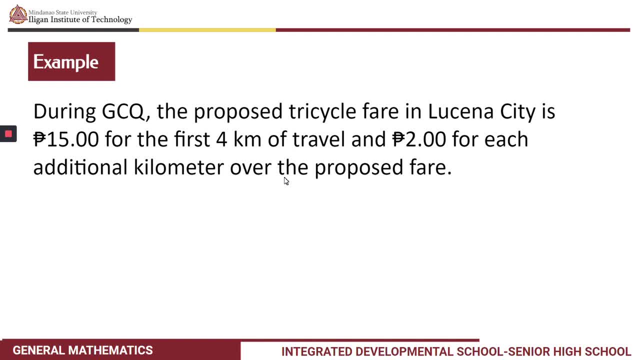 So ang domain dito, or the independent variable is the kilometer over the is the ah the range, It's the ah the distance. no that, that ah a passenger traveled no where the tricycle. 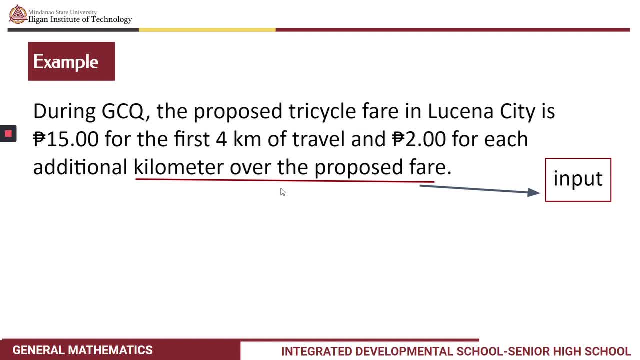 traveled. So yan yung ating independent variable or our domain. So our ah range here is the tricycle fare. Okay, So yan na-identify. na Next is ah You observe yung situation Sabi dito we have 15 pesos for the first 4 kilometers and 2 pesos for each additional. 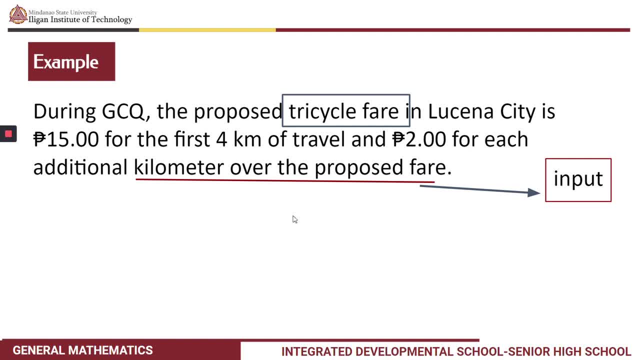 kilometer over the proposed fare. So mayroong dalawang condition. no, If yung destination mo is 4 kilometer or less, you'll only pay 15 pesos. So, kahit 1 kilometer ka lang, or kahit 1 kilometer lang yung destination mo, you'll only pay 15 pesos. So kahit 1 kilometer ka lang, or kahit 1 kilometer lang yung destination mo, you'll only pay 15 pesos. Okay, If you are 현재 tot nga dabayan mahayuran mo, it's okay. It's okay even if you are initially olika. So kahit 1 kilometer lang or kahit 1 kilometer lang, yung destination mo, the same ang mga bayaran mo with the person na magkatravel ng 4 kilometers. 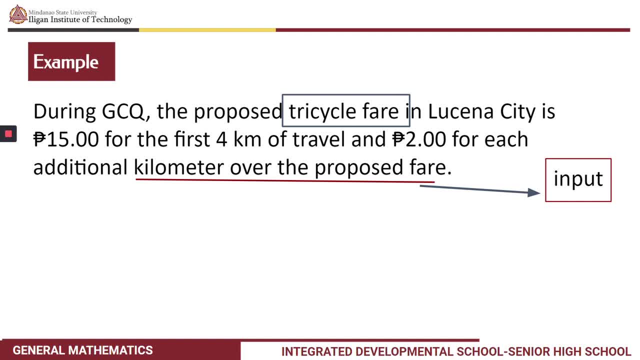 So ayan, yung ibig sabihin ng person statement Tapos sabi dito, is 2 pesos for each additional kilometer over the proposed fare. So if lagpas ka ng 4 kilometers, say 5,, 6, etc. ah, so ma�a-add ka lang ng 2 pesos. 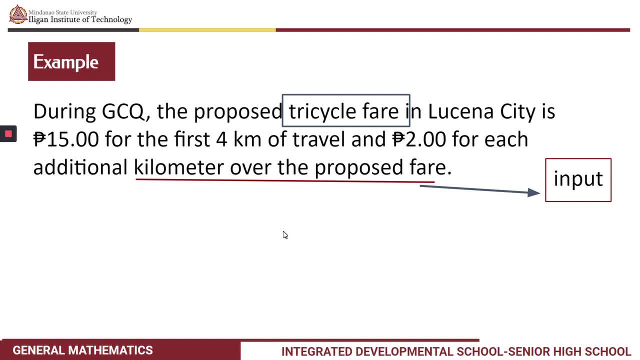 per kilometer naman. Okay, blurr, Kapat ko lang kita here. Okay, So siyempre Good, Okay, auto Ten-e Arkitekt na lumagpas. so for the first one. so our, our piecewise function here is f of x equal to 15. 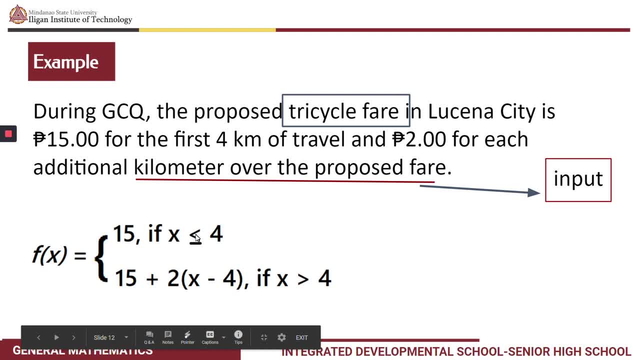 if x is less than or equal to 4, and 15 plus 2 times the difference of x minus 4 if x is greater than 4. itong nasa taas na condition or formula is: if first 4 kilometer travel, yan yung sinabi. 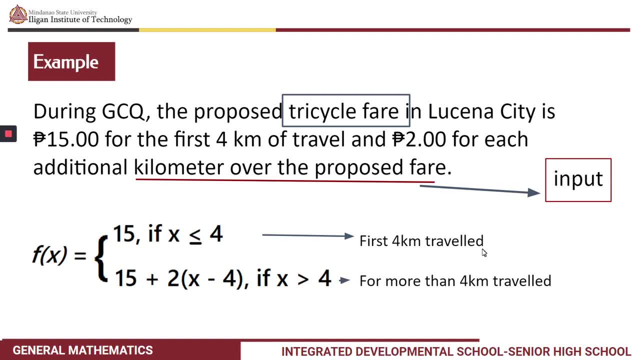 o kanina diba. so 1, 2, 3, 4, 15 pesos lagi yung babayaran. itong pang second naman y x minus 4, y x minus 4, x minus 4, because ang babayaran mo lang na additional na 2 pesos is yung. 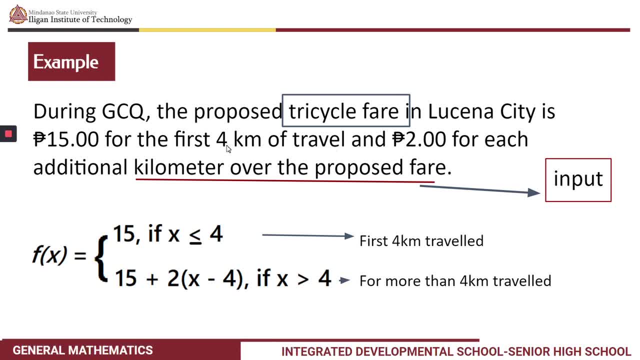 mga lumagpas na kilometers after ng 4 kilometers, so say, for example, um 6 kilometers, so hindi 6 times. uh, you know, hindi si 6, yung magmultiply mo kang 2 para sa additional na fare, ang yung magmultiply mo lang. 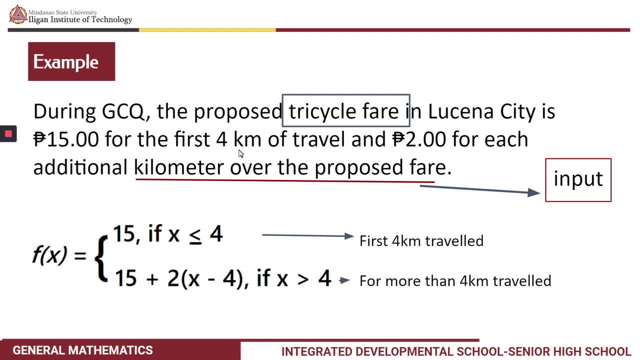 is yung, uh, yung lumagpas na distance, which is 2 kilometers. so yun ang yung magmultiply mo sa 2 pesos, which is the rate for each kilometer. that's why we have x minus 4 here. so that's our piecewise function for this situation, and the domain of course is from 0 to positive infinity. 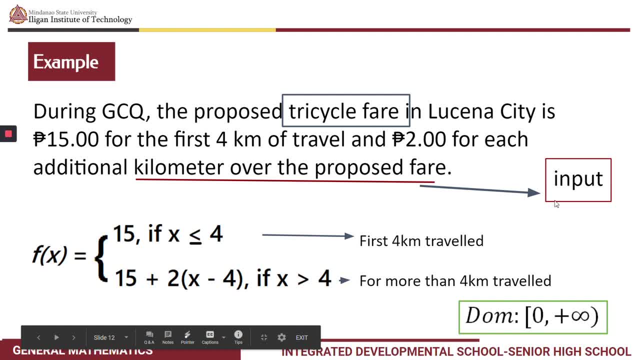 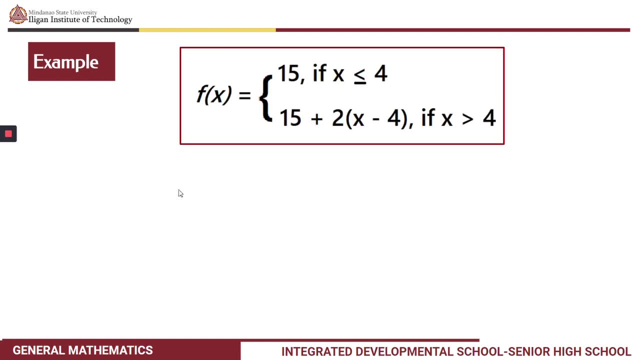 because our input or domain is the distance na na cover and wala tayong negative na distance. okay, so we have this piecewise function, so let's try to solve how much would uh joshi pay if she'll be traveling 10 kilometers? okay, so um sa piecewise function. 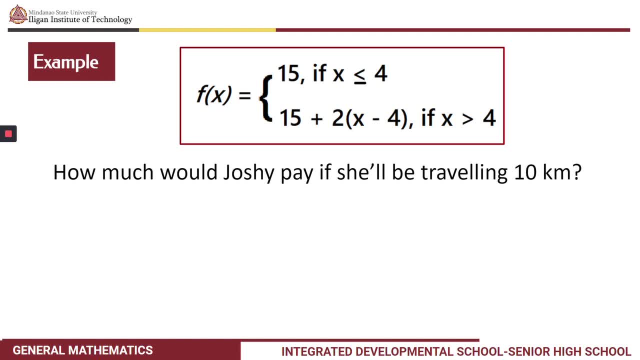 dapat tingnan mo kung saan saan ba na na na na be belong si 10 kilometers, na si 10 kilometers. uh saan siya sa first or sa second second right, because 10 is greater than 4, so that's why we will use the second. so we have f of x equal to 15 plus twice the difference of x. 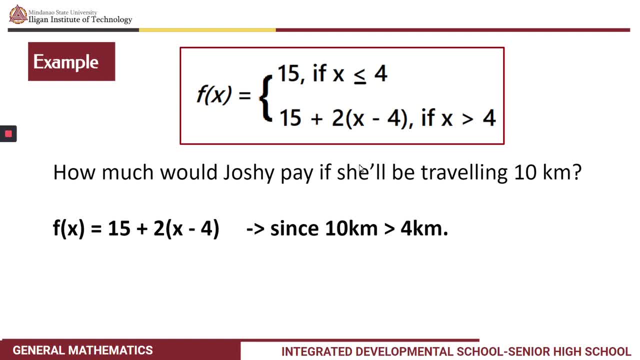 and 4, so substitute tayo ng 10, you have 15 plus 2 times 10 minus 4, so solve accordingly and you will get 27 pesos as a fare, kapag 10 kilometers yung na travel ng passenger early joshi, okay, so ganyan lang. 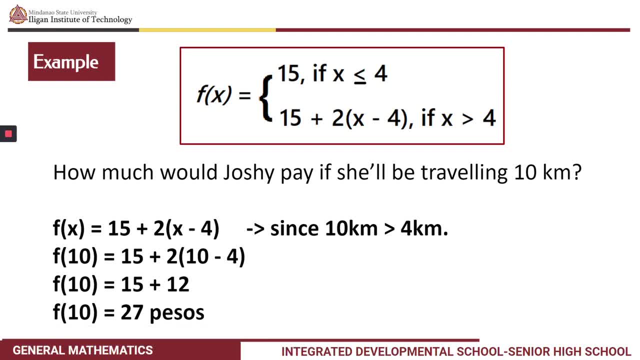 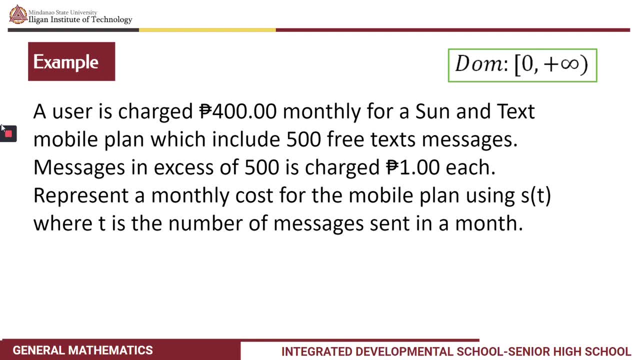 another example: a user is charged 400 pesos monthly for a sun and text mobile plan which include 500 free text messages. messages in excess of 500 is charged one pesos, or one peso each represent a monthly cost for the mobile plan. using s of t, where t is the number of messages sent in a month. ayan, klaro naman kung ano yung domain no. 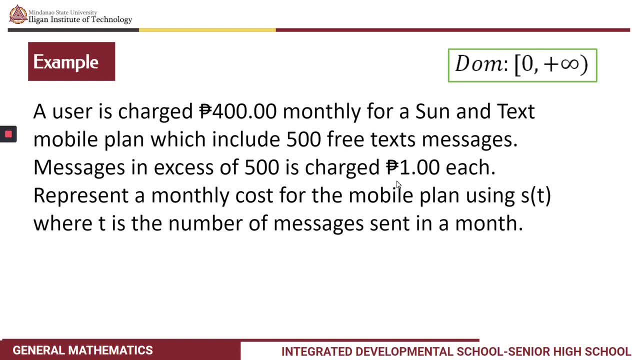 kung ano yung ating independent variable. our independent variable is the number of messages you send in a month and our output, or the range, is what the monthly cost for the mobile plan. so, looking at the situation, mayroon dalawang kundisyon or dalawang. 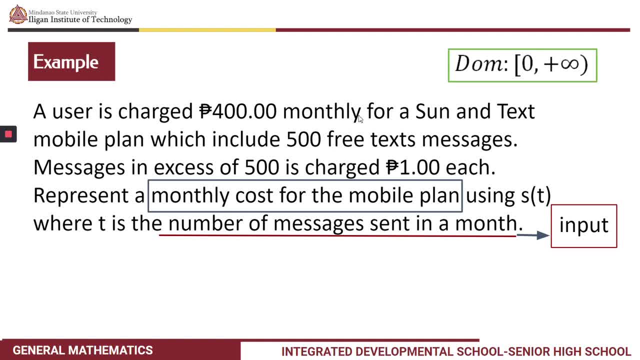 um situation. so first is: if hindi ka na magpaste sa 503 text messages na alotted for 400 pesos, you will get 500 free text messages for 400 pesos, mesages na alotted for 400 pesos na plan. and the second is: if lumagpas ka sa 500 pesos na 500 messages na plan. so 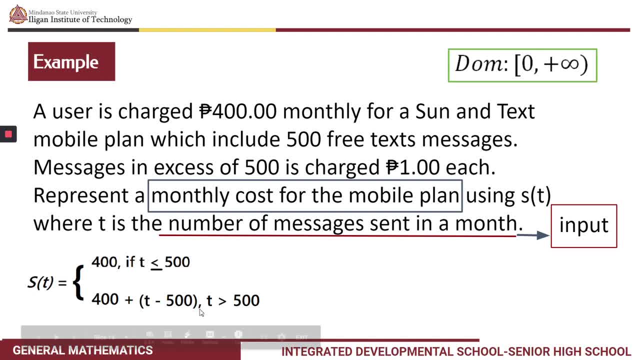 the piecewise function will be 400 if T is less than or equal to 500, meaning 500 text messages or less, and 400 plus T minus 500 where T is greater than 500, which means more than 500 text messages. yung na gamit mo sa in a month, okay, so ang domain pa rin dito is: 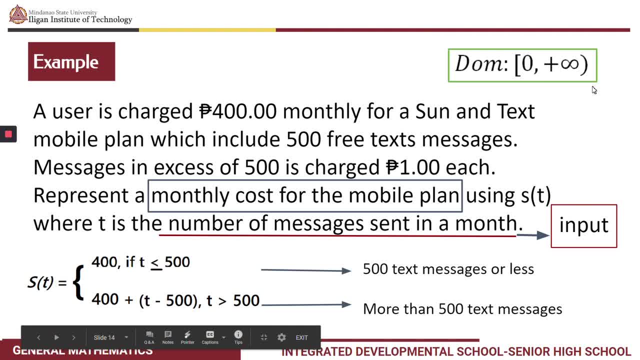 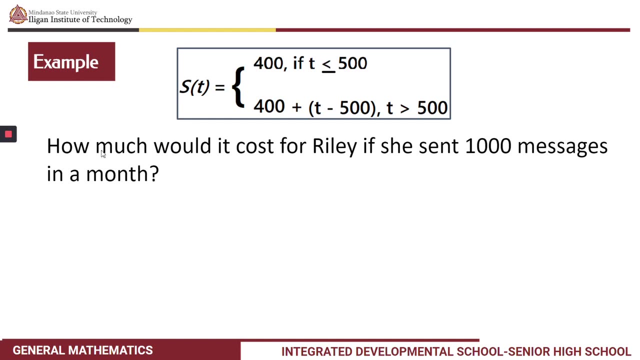 from zero to positive infinity, because our or you can set our yung base wan bit per month when we plot negative number of texts, messages. so let's try to solve if. how much will it cost for Rie Lee if she sent 1,000 messages in a month? so again, ang gagawin na natin is mag-substitute. so we have 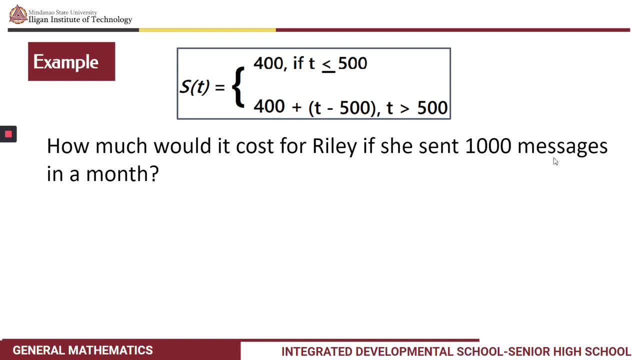 emic. substitute: see 1,000 messages. of course, a second now, because T, which is 1,000, is greater than 500. so that's why we'll use this second formula or equation, which is S of T equal to 400 plus T minus 500. next thing to do is to substitute 1,000. okay. 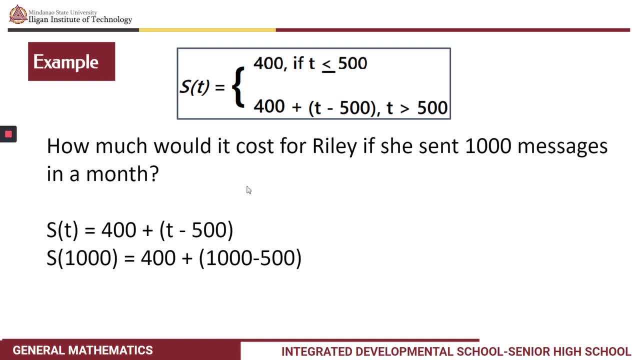 so you'll have S of 1,000, equal to 400 plus 1,000 minus 500, and if you solve it accordingly, you get 900 pesos. so that is now your cost, or what will you pay if you will send 1,000 messages, if you pass the 500 messages of the plan? 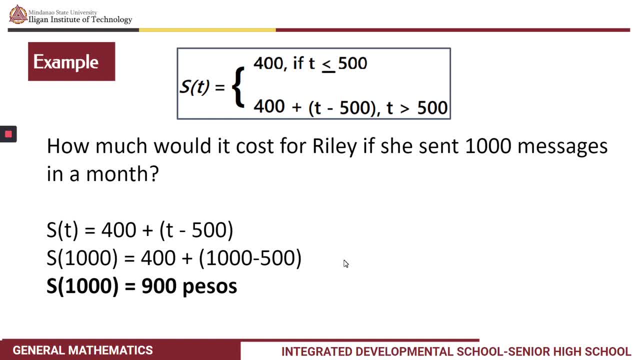 okay, so this is our representation of functions we have. first, we need- really need- to get the domain and the range first, but we know which one is input and the output. after that, observe the situation, if it is applicable piecewise or not, and then generate your function rule and that will be the function model of the real life situation. so I